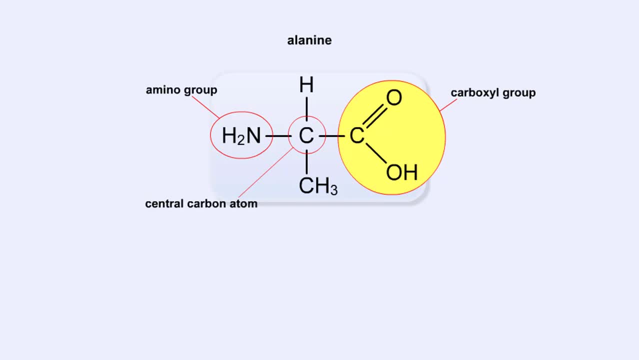 This is where the carboxyl group gets its name. carboxyl- The carboxyl group is attached to one of the oxygen atoms- is what gives the amino acid its acid properties. The final two groups are easy. The first is a hydrogen atom that is bound to the central carbon atom. 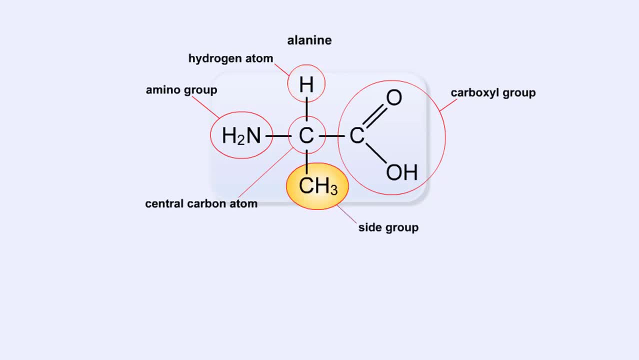 The second is the side group, which we discussed earlier. The side group is different for each amino acid and it will affect how the amino acid acts when it binds to other amino acids. So let's take a look at how amino acids bind to each other and make proteins. 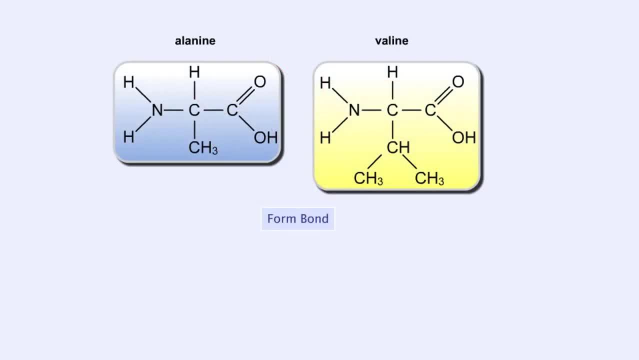 The bond between two amino acids is called a bond. The bond between two amino acids is called a peptide bond. Now let's look at how these bonds are formed. When a peptide bond forms a molecule of water is produced, Which atoms in these two amino acids do you think might be lost to form this water molecule? 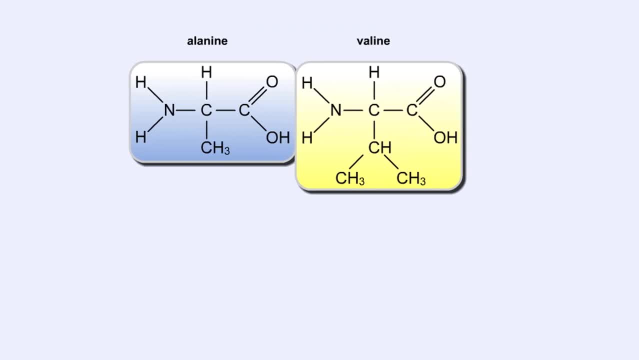 Watch this peptide bond form between alanine and valine. The carbon atom in the carboxyl group of alanine reacts with the nitrogen atom in the amino group of valine. The carbon atom in the carboxyl group of alanine reacts with the nitrogen atom in the amino group of valine. 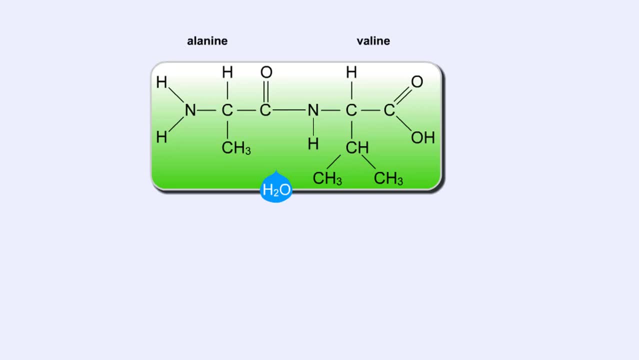 At the same time, the alanine loses an OH group and the valine loses a hydrogen atom, forming the water molecule. This kind of bond is repeated within a protein thousands of times using many different amino acids. In a living cell, these bonds are created in a set order, for each protein on a cellular structure called a ribosome. 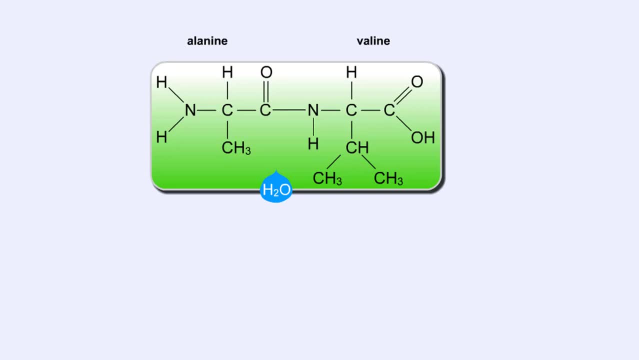 But that will be discussed in detail in a later animation. Right now, let's take a closer look at the central carbon atom and how it affects the whole protein molecule. The central carbon atom is the point at which the other parts of the amino acid rotate. 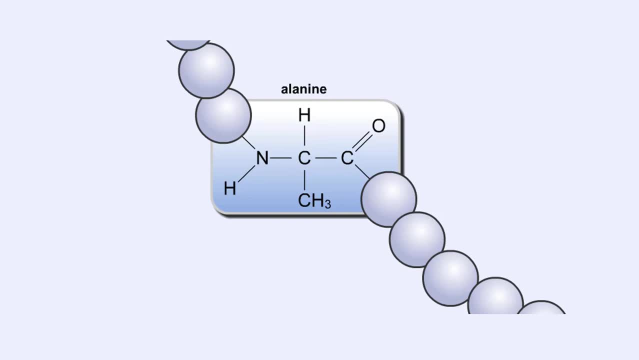 Small rotations of the bonds around the central carbon atom can lead to large changes in the overall protein structure. When you have a protein with thousands of amino acids, these small rotations can add up to a large variety of complex structures.